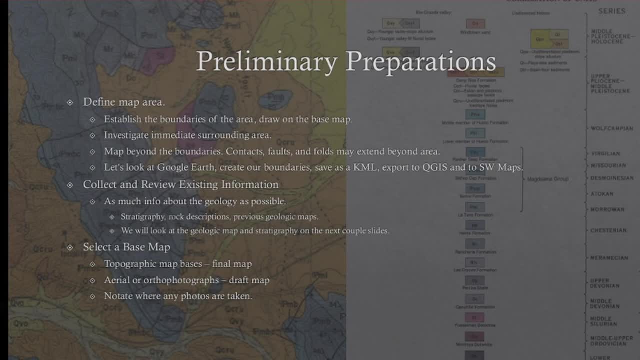 immediate surrounding area. you map beyond the boundaries, which includes faults, contacts, folds, which may extend beyond your area, and then we're going to look at qgis. but you can use google earth as well to create your boundaries. so you save it as a kml and export it to qgis and then i use 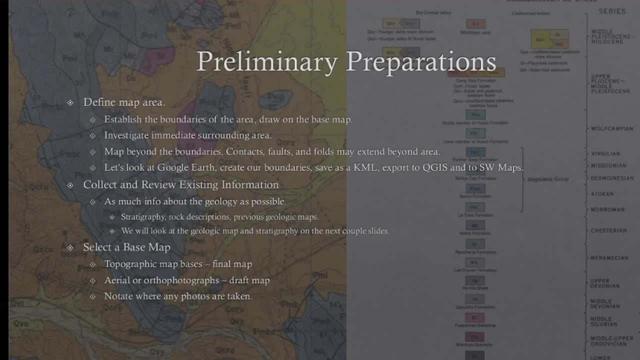 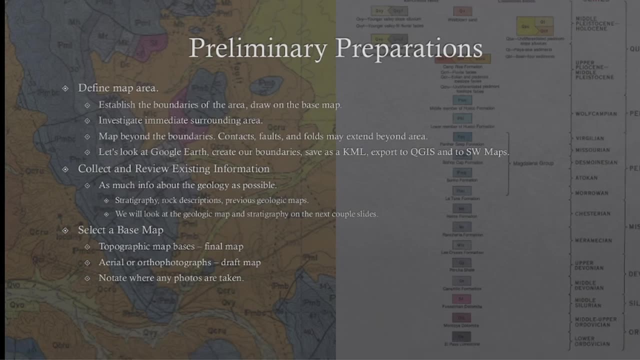 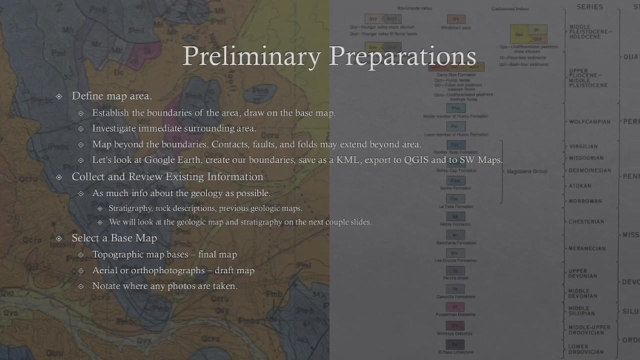 what's called sw maps. it's an android app that you can use to do some mapping on a q field is probably better. i should say we didn't really map when we went out for our field work, just kind of enjoyed the hike. but i plan on building on this eventually and q film and doing. 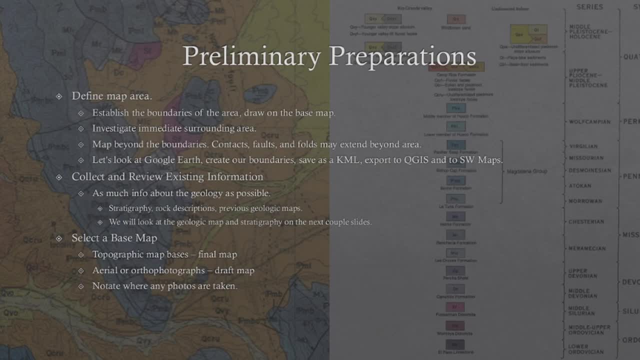 an actual map on my phone, so for this instance. so we're going to collect and review existing information, as much information about the geology as possible. so you want to research the stratigraphy, the rock descriptions, the previous geologic maps. we'll also look at the geologic map and stratigraphy. 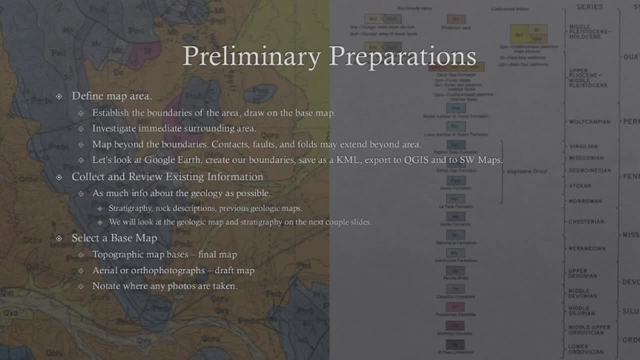 on the next couple slides and you got to select a base map. use topographic base map for your final map, but for your draft map you can use an aerial or ortho photograph and then notate where any photos are taken. i like to a combination of both. for the final map, the aerial mixed in with a low. 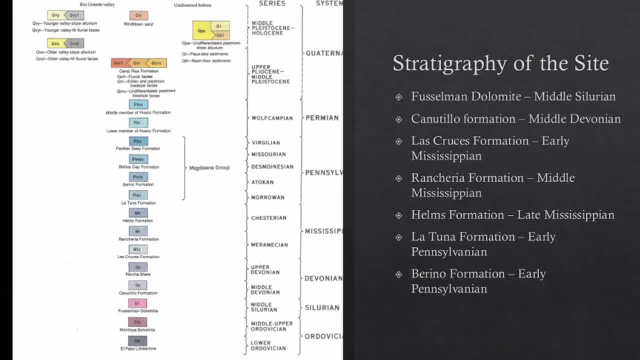 lower opacity of topographic map. so the stratigraphy of the site. you have the fussaman dolomite, which is middle salarian, and the theo middle devonian, las cruces, early mississippian rancheria, middle mississippian elms, late mississippian latuna and barino, early pennsylvania. so, as you can see, starts here. 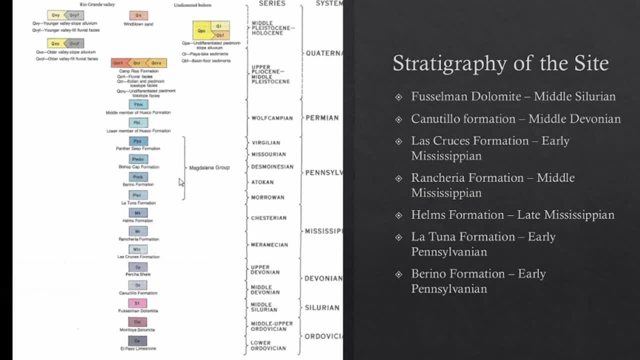 yeah, the solarion all the way up into the early pennsylvania. right here, barino is one of the rocks that we'll see when we get the saudia at the end of that trip, when it gets to the south of the United States- see in the video- we'll also see the bustleman dolomite as well. those are the two rocks that. 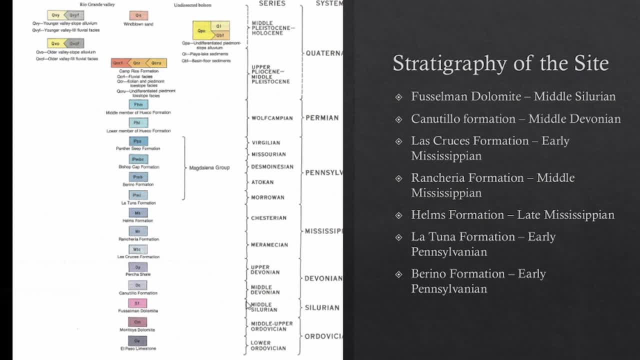 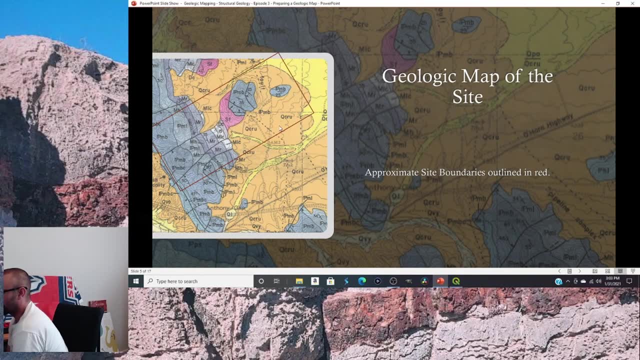 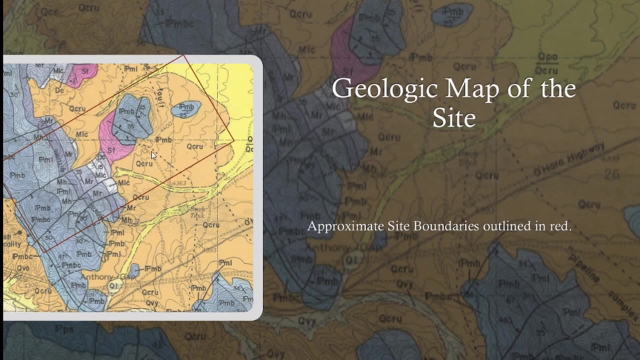 you'll see in during the uh, the filled portion of this video. i created my map. this is a geologic map that's been performed on the site before. it's technically good to look at that and kind of prepare yourself to uh, to what your you'll be, um, what you'll be uh. 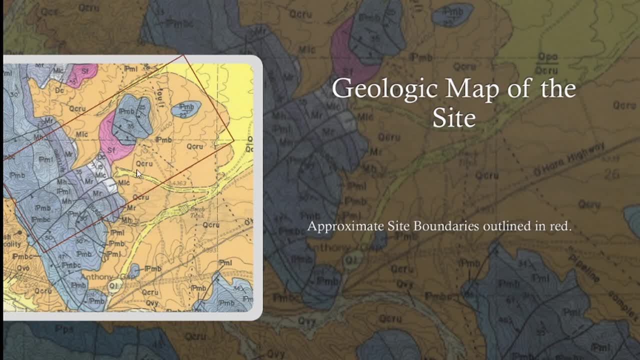 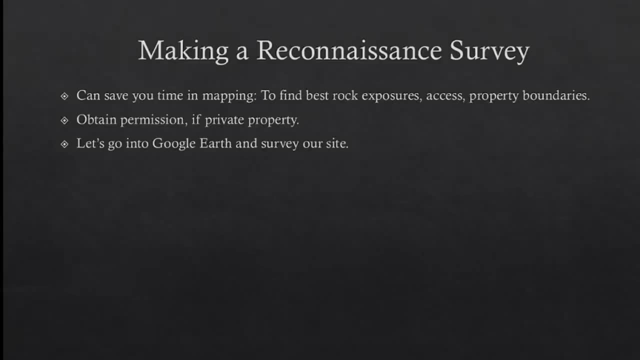 mapping: go to the site, type of rocks you'll be looking for, what type of contacts you'll be looking for. making a reconnaissance survey, which can save you time, and mapping: you want to use this to find the best rock exposures. access property boundaries: you have to obtain permission. if it's private property, you don't want to get shot and 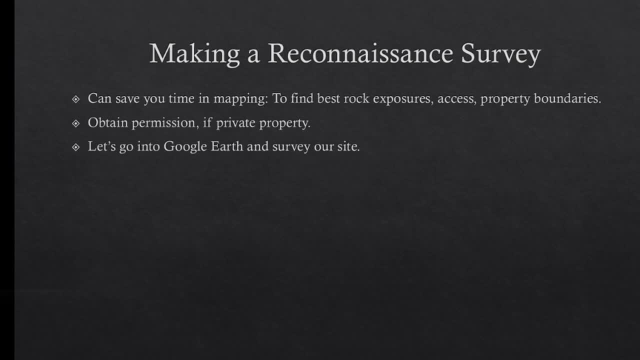 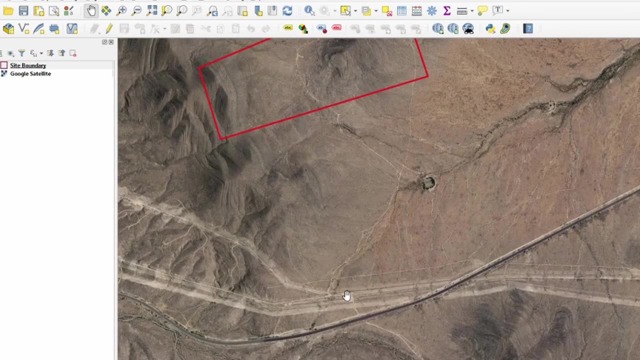 let's go into qgis, not google earth. survey our site real quick. so this is our site. we already did our field work, but we drove on this road. we'll go right right here up to here, took a left, came up here. actually we stopped right about here. there's a washed out. 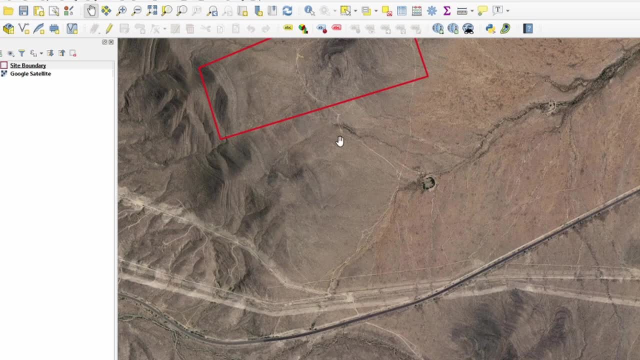 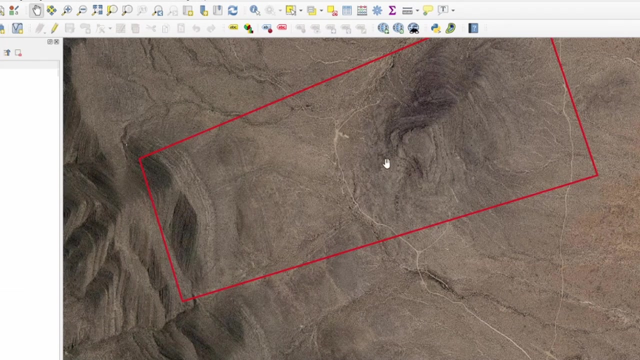 uh, the road is washed out right here, so you'll die if you go any further than this, unless you have a motorcycle and you could travel this way. this is our site boundary, as you saw on the geologic map. you know this is a little valley. got your high elevation right here and then. 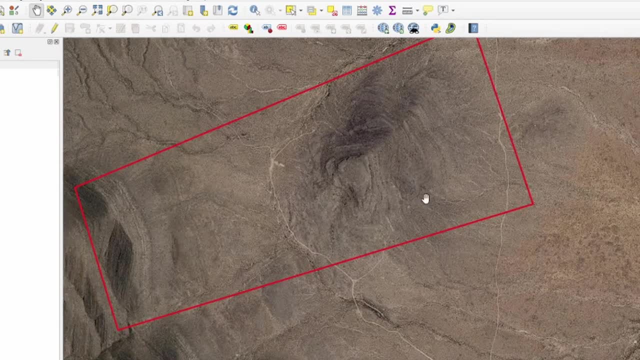 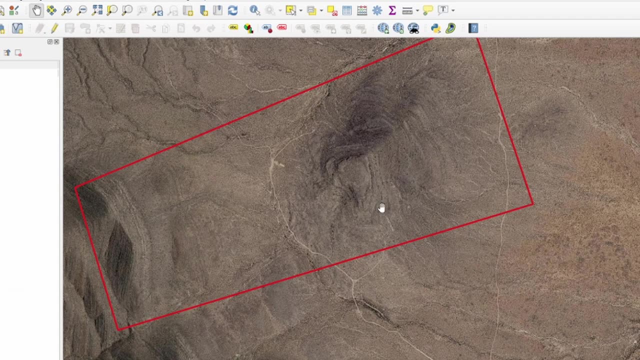 right here. it's a pretty simple site. bustleman is right here. oh, fussman's actually down here. then you have the barino, which i'll, as you'll see in the video, those two should not be in contact with one another. that tells you something. it's a fault contact. and then, as you trek this, 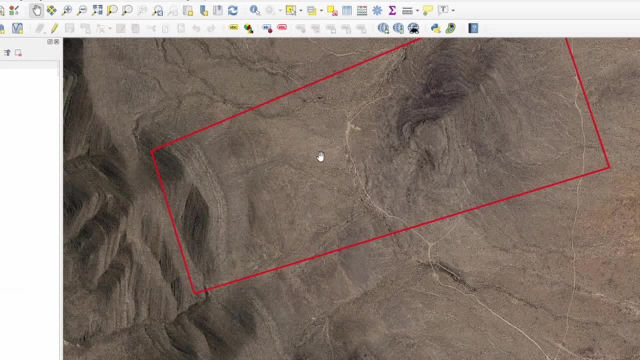 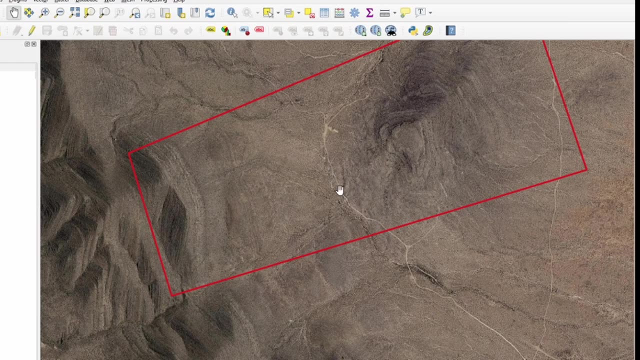 way. you go into basically the stratigraphy in the right order. so as you walk up you're going into you'll you have the fossil men. go into rancheria, then las cruces or kennethio, then las cruces and then the helms and latuna and barino. you know it's in order, so there's no faulting. 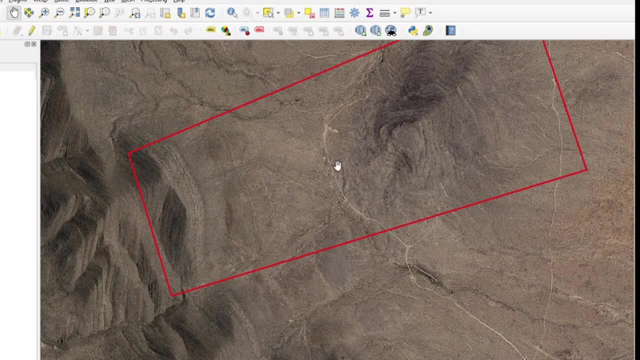 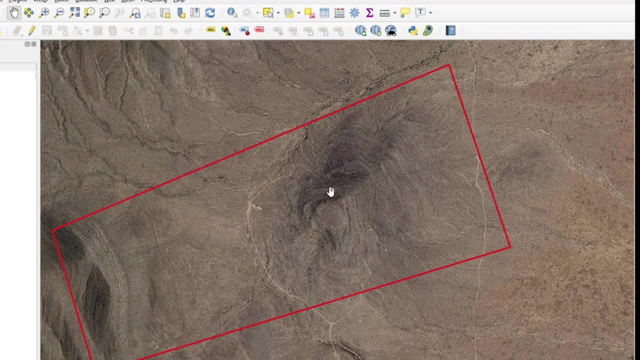 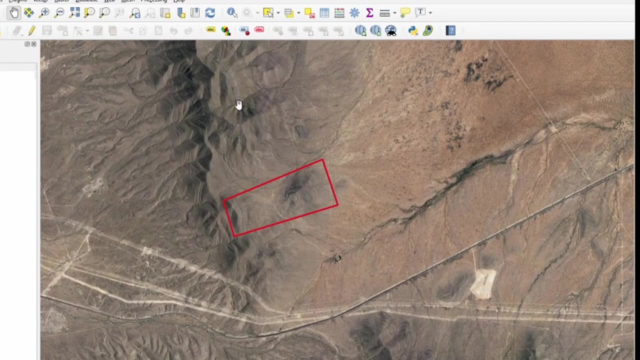 there are unconformities here and there but, um, you know, there's no faulting in this particular portion of the site. faulting there's two or three faults that cross cut and specifically this fault here comes back over here, as you can see a little bit displacement on the beds right here. 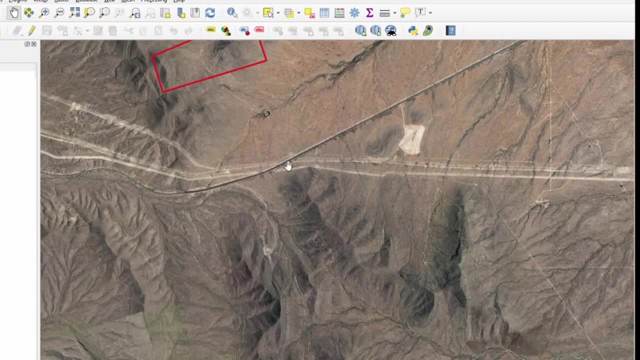 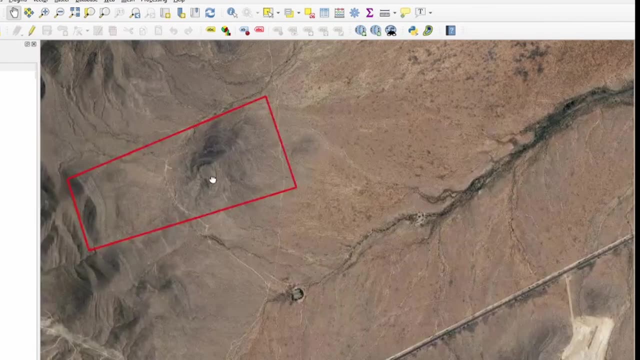 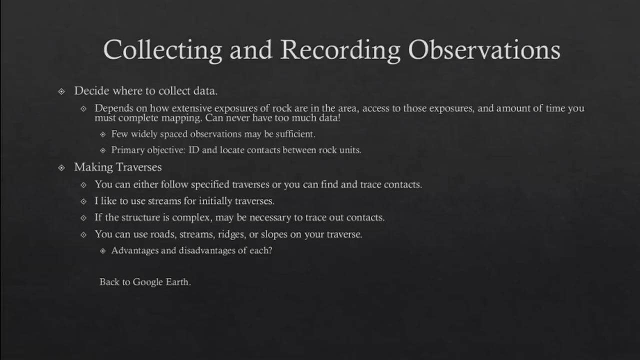 then the fault cross cuts this road, this access road, this big road. here i've actually mapped this area for field camp. i didn't map it this time, i think eventually i would like to so collecting and recording observations. decide where to collect data depends on how extensive exposures of rock are in the area. 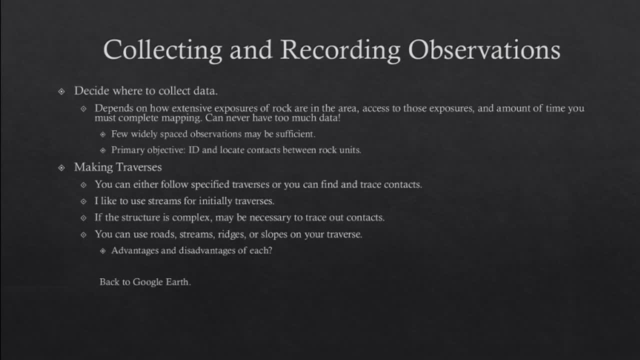 and the amount of time you must complete the mapping, and you can never have too much data. few, widely spaced observations may be sufficient. so you don't want to take a bunch of strike and dips in one area and or the rest of the area. you want to kind of spread out your strike and dips. 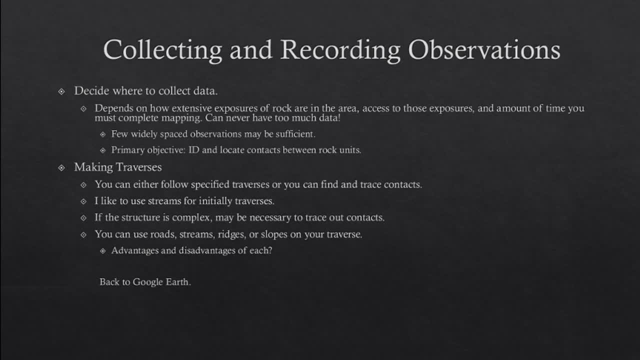 your primary objective is to identify and locate contacts between rock units you're when you're making your traverses. you can either follow specified traverses or you can find a way to trace contacts. for me personally, i like to use streams, initially on my first day, and use those to map where contacts are, and then, the harder you know, the more difficult hiking. 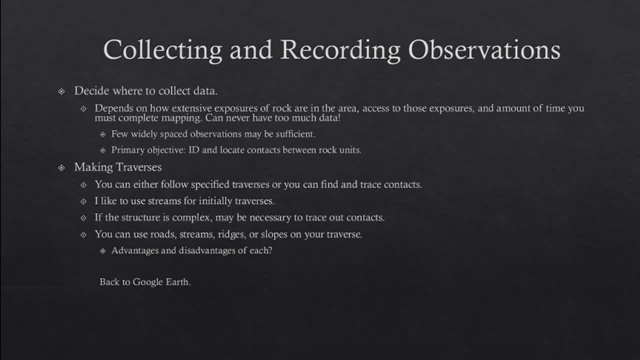 and mapping portions i'll save for the next day or the the day after that, depending on how much time you have. i only had one day and it was only like four hours, not enough time to map the entire site anyways. but and if the structure is complex? 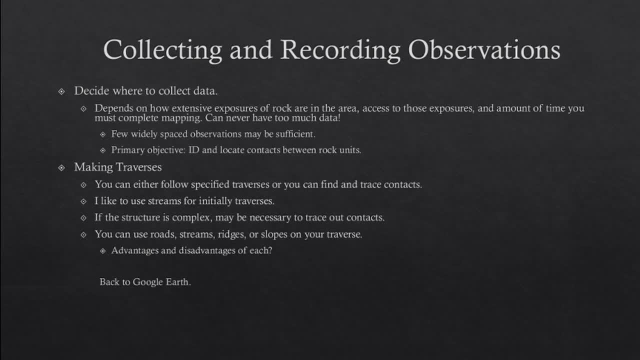 it may be necessary to trace out the contacts. so in that area i was talking about where Barino and Musselman are in contact- you'll definitely want to trace that contact further than i did. that you'll see in the video. you can use roads, streams, ridges or slopes on your traverse. 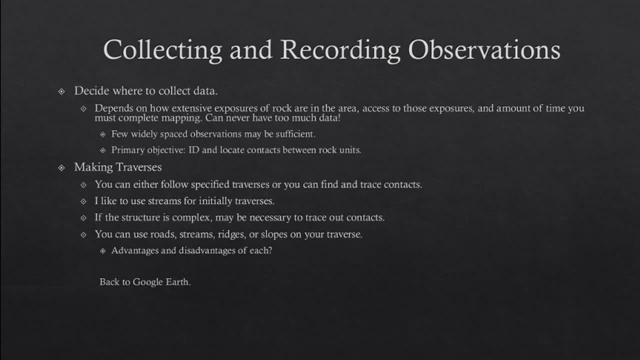 think about the advantages and disadvantages. disadvantages of each roads. will those take you to good outcrops? probably not streams. they are good to find the contact points or the contacts between rocks, but they're not good for taking strikes and dips, something you have to think about. ridges: 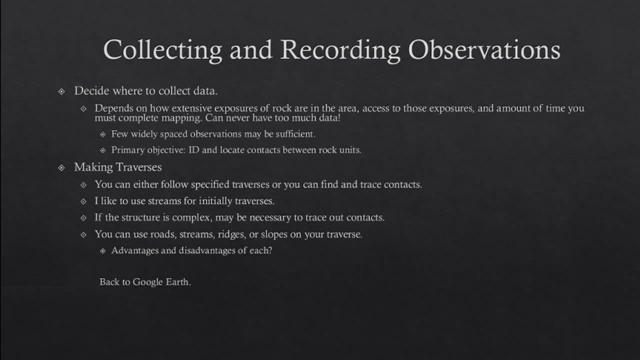 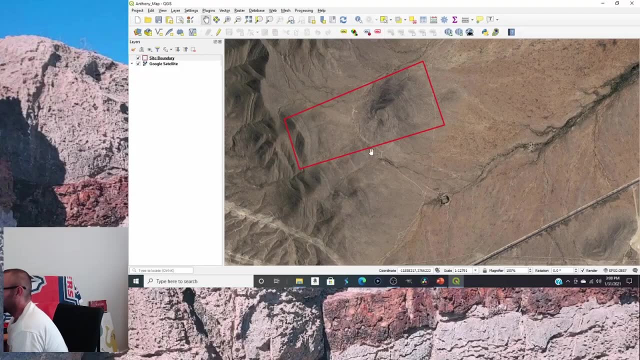 good for strikes and dips but difficult to hike up. same with slopes. obviously, ridges you you can't really hike up unless you find a other avenues. the traverse that we did: walked across this, parked here, walked across this, went around and came up here to look at the ranch area. I did not include in the 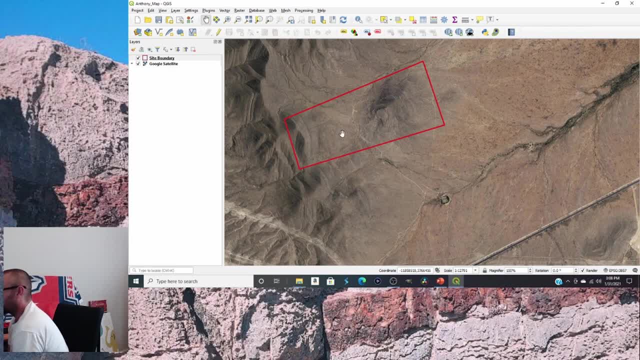 video, I will definitely be talking more about sedimentary rocks, which all the rocks in this area are sedimentary. we're gonna be talking about scribing sedimentary rocks. I want to return to this site and use that episode to talk about how to describe sedimentary rocks and when you're collecting and recording. 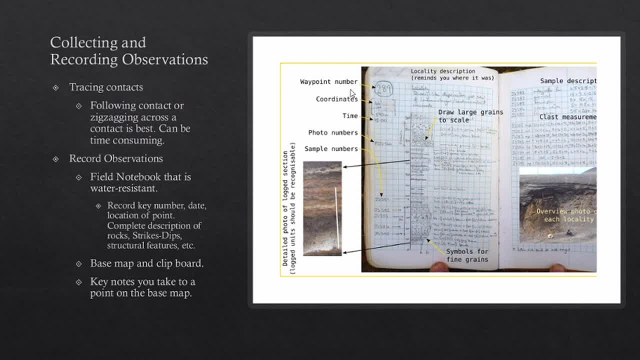 observations. you obviously want to know how to describe sedimentary rocks and to have your field notebook, as you'll see on the right side. you want to trace your contacts. you can either follow the contact or zigzag across a contact and obviously these can be time-consuming. you kind of for me, I just walk up and 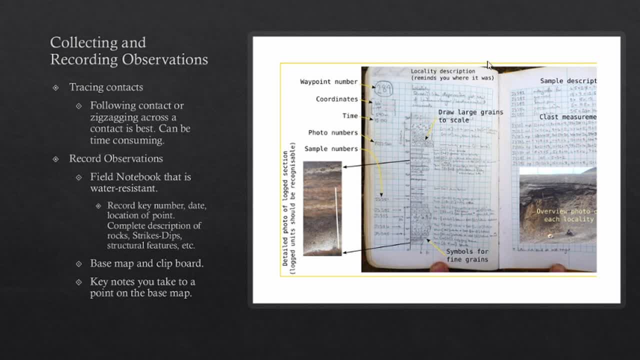 mark where contacts are as I, as I go up, and then when I'm coming back down, I'll like a stream down a stream. I'll mark the contacts again and then just connect the points and, as a rough draft, that's all I'm going to do is I'm just going to 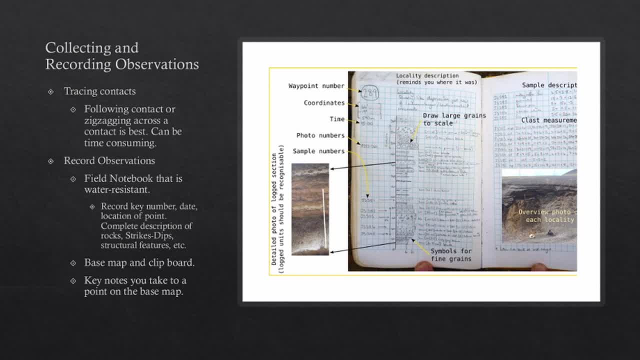 step back and Subtitles by the Amaraorg community: structural features, etc. I like to use waypoint numbers. You know, on your paper map you mark a one and that can be, you know, a certain rock that you see, that you did a stratigraphic column. 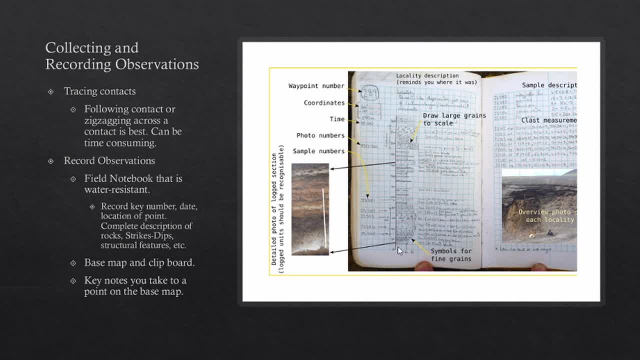 for, for example, And obviously that's their stratigraphic column right here. That's a good way to create a description for a sedimentary rock And you mark it on your paper map and you can basically key it in your fill notebook and tie it to your paper rough draft map You want to. 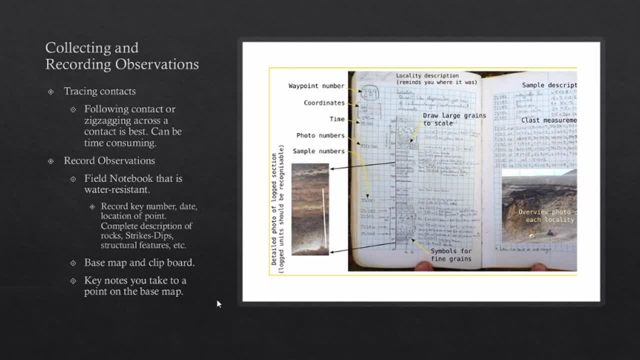 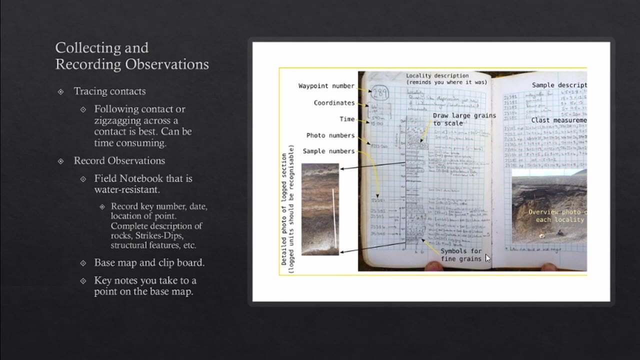 have your base map and clipboard and you want to have keynotes you take to a point on the base map, like I talked about, And if you have a GPS on you, which we all have phones, so you can record your GPS, your time, if you take samples, sample numbers, symbols for final fine grains, clays are going to. 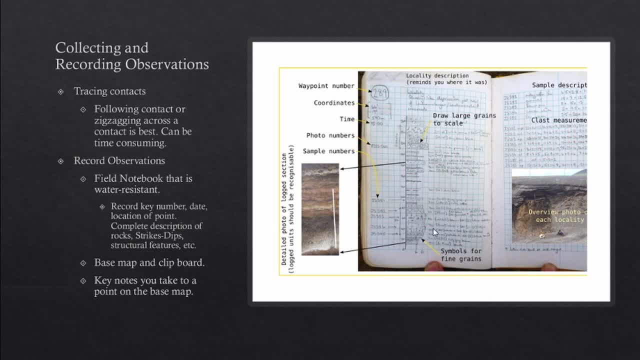 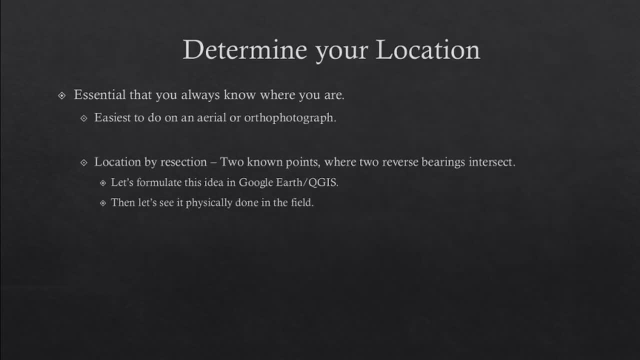 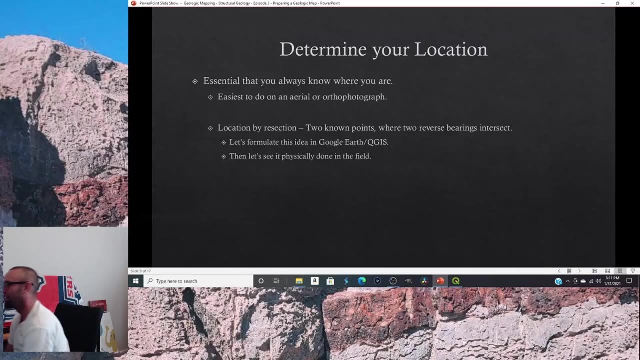 have the little dashes Symbols, whereas sands are going to be bigger. specs and so on and so forth. Pretty detailed fill notebook- I wish mine looked that good- And determining your location. it is essential that you always know where you're located. With GPS it's easy to to kind of know where you're located. 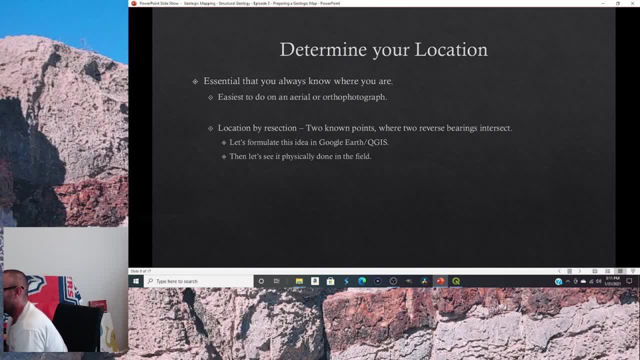 And it's easiest to find yourself on an aerial or ortho photograph. One way to do it when you don't have your technology is to do location by resection. Take two known points where to reverse bearings intersect. So you gotta have a paper map and you gotta have your protractor with. 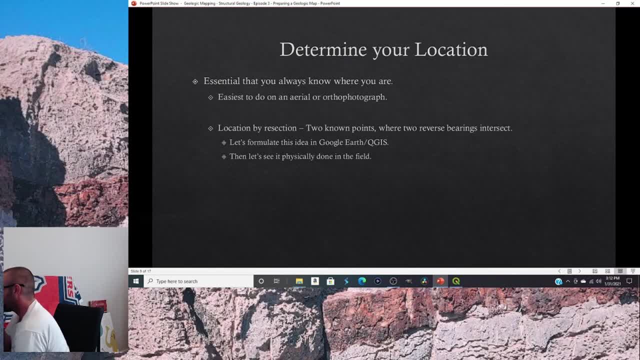 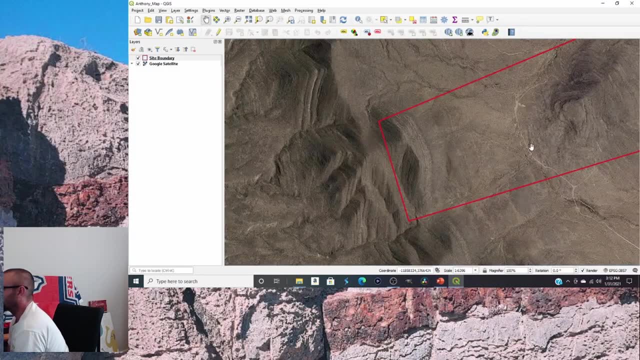 you. So let's formulate this ID in Google Earth, And we're not gonna see it done in this episode. maybe eventually I'll do it. But let's say we're right here in the middle of this road And we want to know. 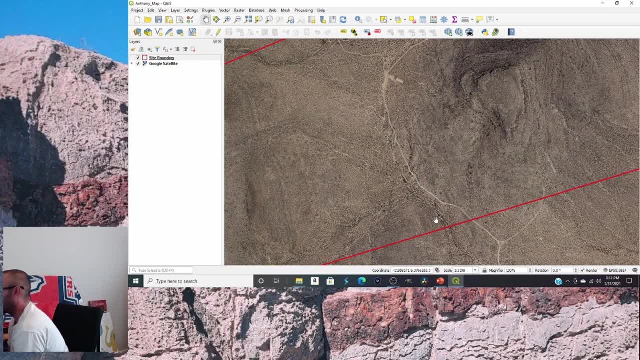 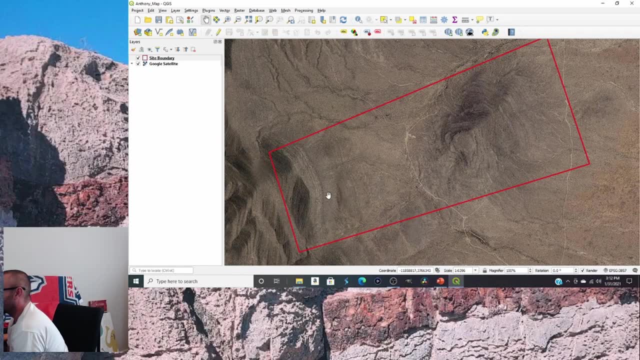 where we are, which obviously we are on a road, so you should be able to know that where you are. but anyways, you're right here and you want to shoot with your brunton a bearing towards this point. there's a high point over here somewhere. shoot it towards that point and then. 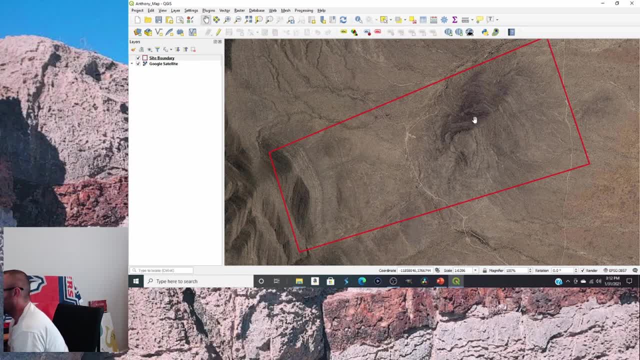 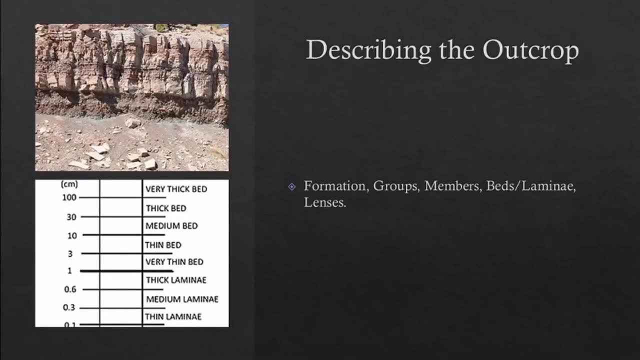 shoot a bearing towards this point and, with a protractor, take that angle from that point that you shot at and measure it over here. wherever the lines intersect, that's where you are located. it's called location by resection and then describing the outcrop. i want to make sure 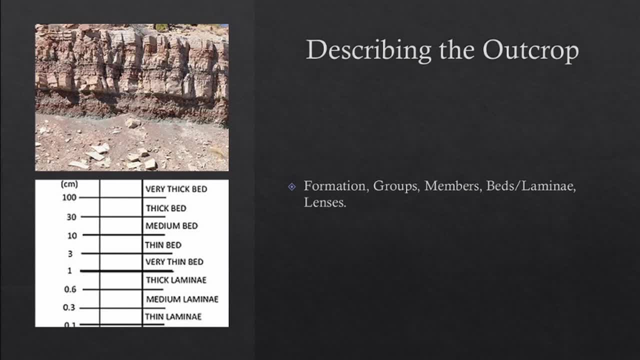 that you're describing your outcrops significantly and that leads into the next episode. but you have formations, groups, members, beds, laminate and lenses. so when you're doing what's called a stratigraphic column to create a great description of, well, these are all carbonate rocks, sedimentary. 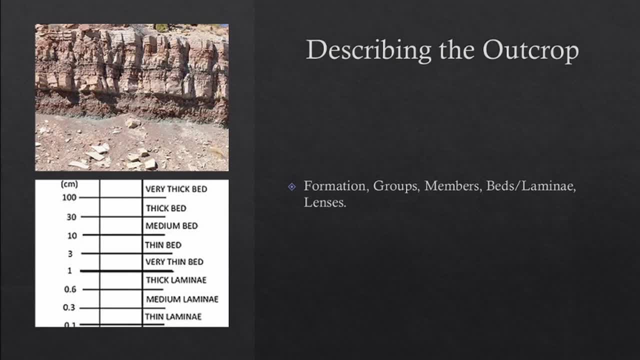 carbonates. stratigraphic columns are such a great way to create a beautiful description of the outcrop, and then you're going to take a shot at that point, and then you're going to have very thick beds, as you can see on this chart over here, to thin laminate anything above. 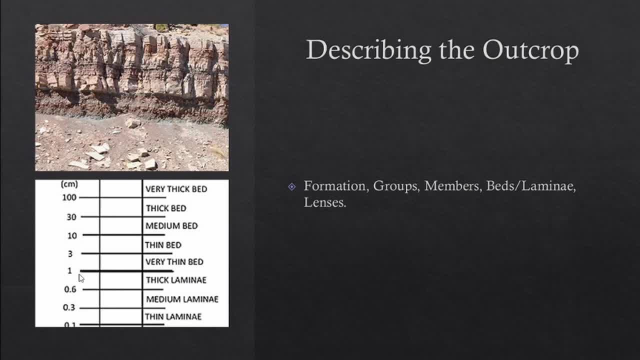 one centimeter is considered a bed and below centimeter is considered a laminate, just so you know. and then lenses are just thin, discontinuous beds. so they'll just literally be a lens trapped in, say, a carbonate. you'll have a chert lenses and some of these carbonates that, uh, that you see at 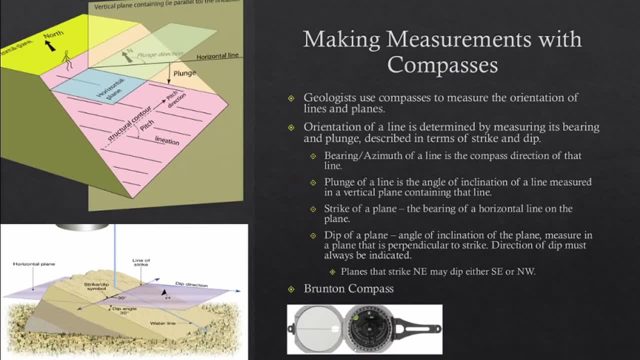 the bottom here are made of carbonate. that's 거� you use bearing and plunge to measure the fold axis or a fold in general. Measure the characteristics of the fold, Use those and the strike of a plane is the bearing of a horizontal line on this plane. 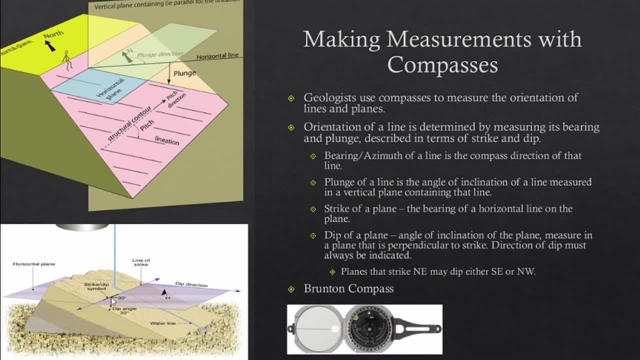 So you can imagine, this is your strike on this rock layer and it's dipping this way Wherever. if you drop water on the surface, wherever it flows down, that's the direction of your dip. Dip of a plane is the angle- angle of inclination of the plane, measured in a plane that is. 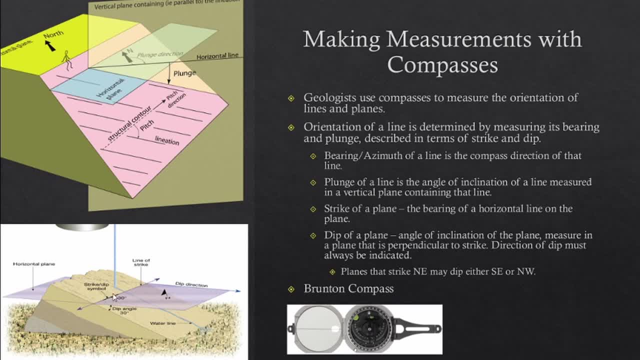 perpendicular to strike, which is important. Your dip is always perpendicular to your strike line and the direction of dip must always be indicated. Now, planes that strike northeast, which is what this is striking. Let's just say: this is north, this is northeast. It may dip either. 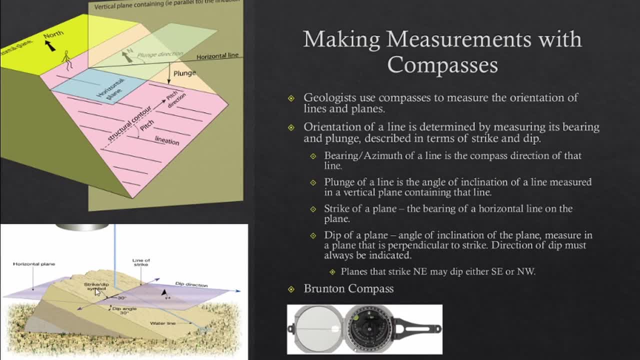 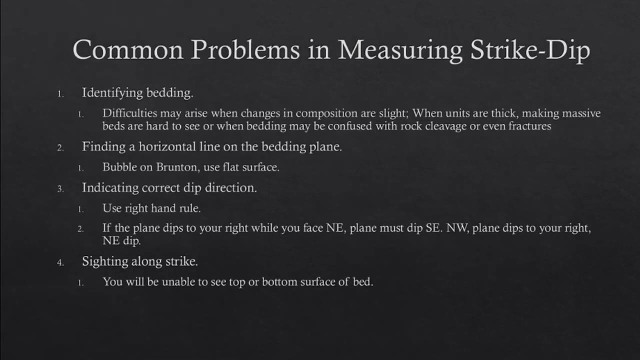 southeast or northwest. So it could. it could dip this way, obviously not with this bed, not with this rock, but this one is dipping southeast in this case. Common problems in measuring strike and dip. Identifying bedding Difficulties may arise when changes in composition are slight, When units are thick, massive beds are hard to see, or when 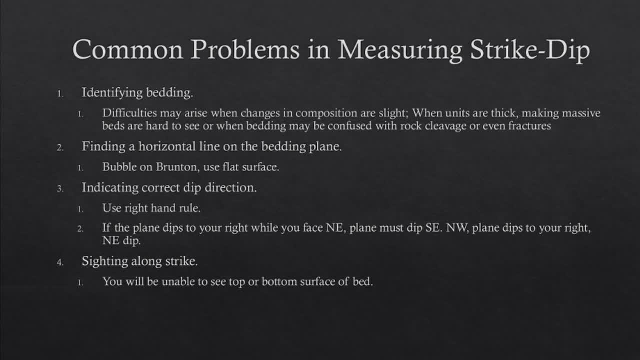 bedding may be confused with rock cleavage or even fractures. When I was early in my geologic education I definitely struggled with understanding what bedding planes looked. I would confuse them with fractures. Finding a horizontal line on a bedding plane, The bubble on the Brunton can be used and make sure you use a flat surface. 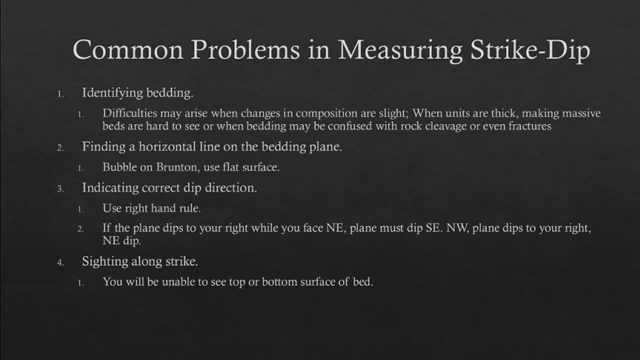 On the rock you're trying to measure. strike and dip on. indicate your correct dip direction. Use your right hand rule: If the plane dips to your right while you face northeast, the plane must dip southeast. Northwest plane dips to your right, northeast dip. Siding along the strike you will be. 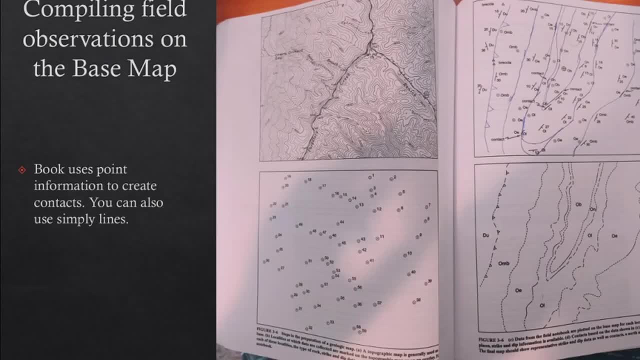 unable to see the top or bottom surface of a bed. Compiling field observations On the base map- the book uses point information, as you can see on this page right here- Then they, you know they- collect this data and then when they get back from their field mapping they'll. 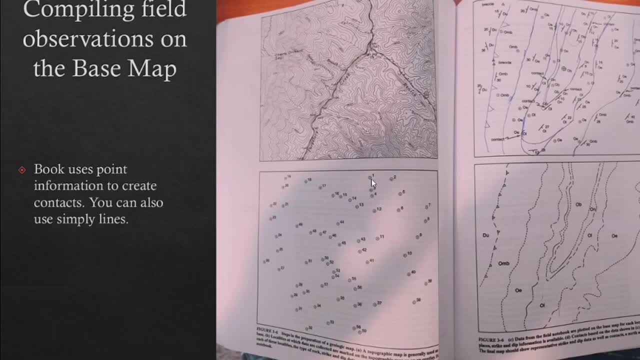 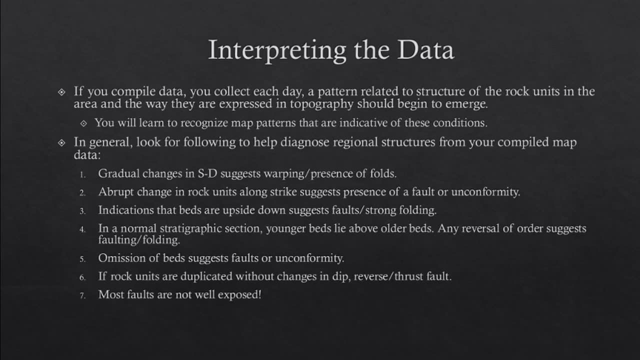 just connect the points. They'll have this keyed in their field notebook. To me, it's easier to just do the lines in the field, Interpreting the data. If you compile data you're going to collect, you collect each day a pattern related to the structure of the rock units in the area and the way they 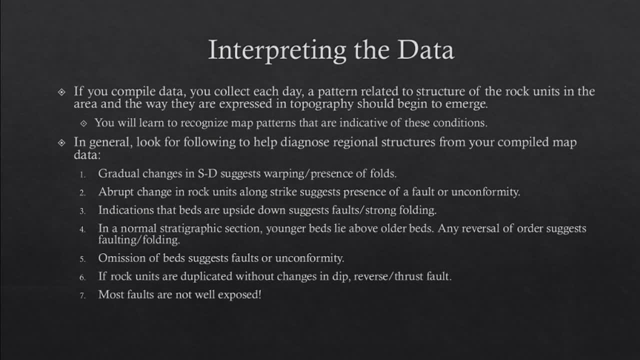 are expressed in topography should begin to emerge. You will learn how to do that in the future. You will learn to recognize map patterns that are indicative of conditions General. look for the following to help diagnose regional structures from filed map data: So gradual. 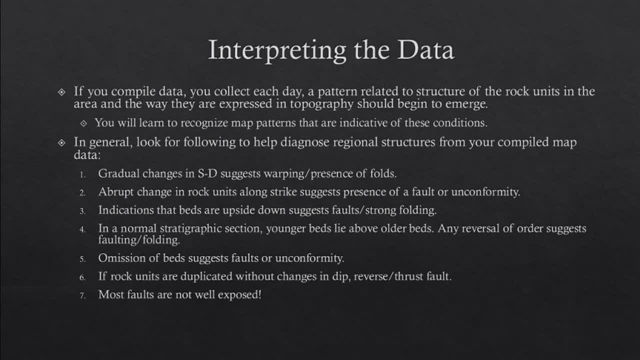 changes in strike dip suggests warping or presence of folds. Abrupt changes in rock units along strikes suggest presence of a fault or unconformity. Indications that beds are upside down suggest faults or strong folding In a normal stratigraphic section younger beds. 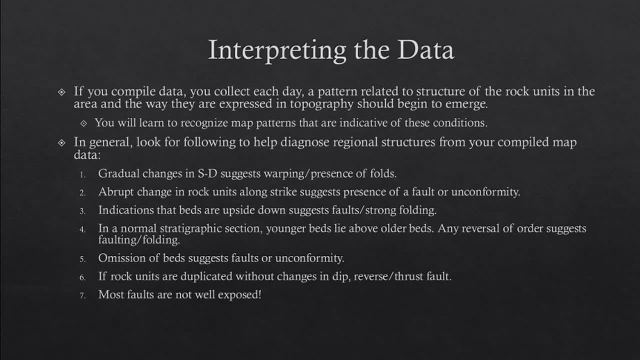 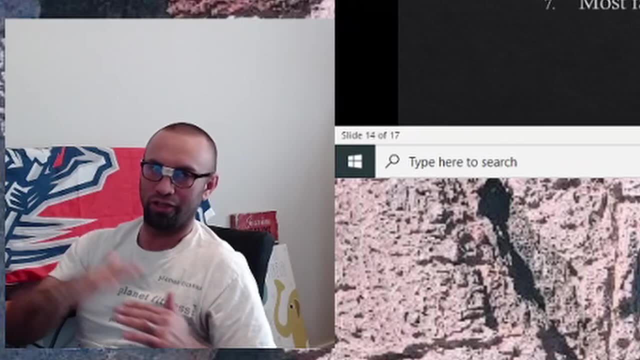 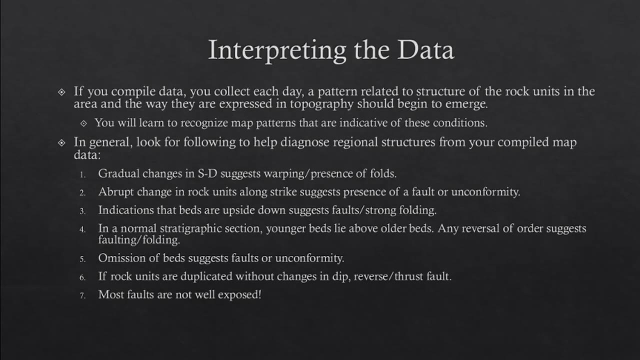 lie above older beds. Any reversal of order suggests faulting or folding. You'll see in the video that we have burino fossil mint Anywhere near each other in the stratigraphy large fault putting somewhere through those two. The omission of beds suggests faulting or unconformity, Like I, 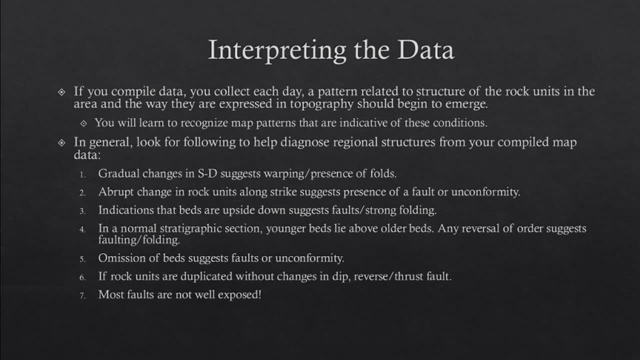 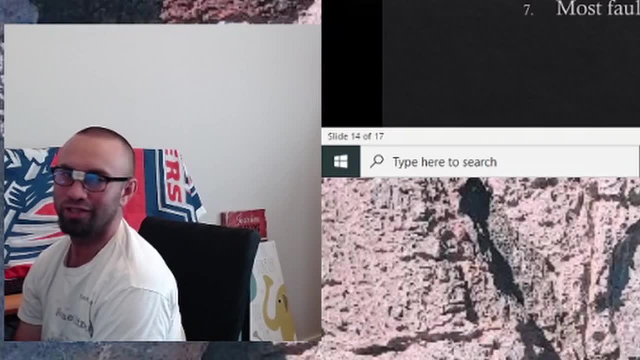 said, if rock units are duplicated without changes in dip, it's a reverse thrust fault and most faults are not well exposed. and the fault that you'll see in the video is not that well exposed. It's a very old fault and eroded, but you can tell by. 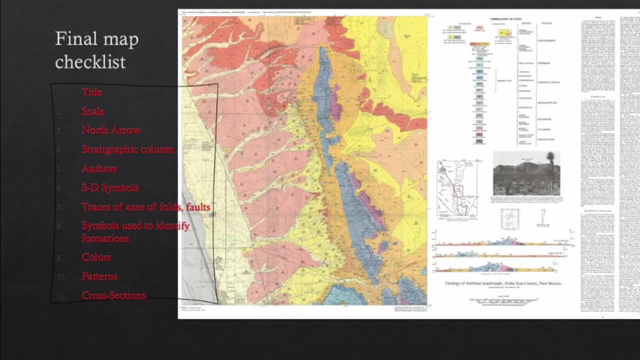 identifying the rocks For your final map checklist. you want to make sure you have your title down here. Theology of Anthony Quadrangle: do shore Doñana county in New Mexico Scale, which is right here at the bottom. you're not going to be able to see it. it's not zoomed. 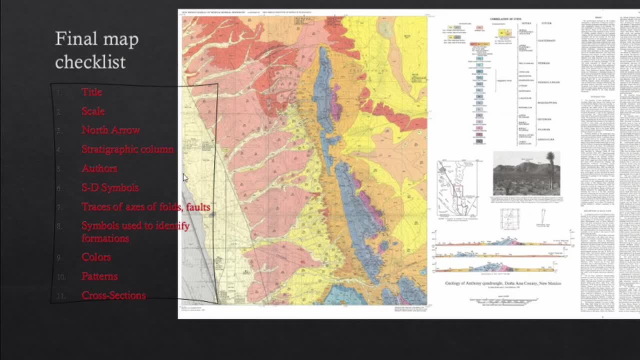 in enough. North arrow is right here. The stratigraphic column is here in this area. Your author is D honey. Не Much Something. Brockummer is here as well. Shieisiertz blandcommereuf lucané before solstice. 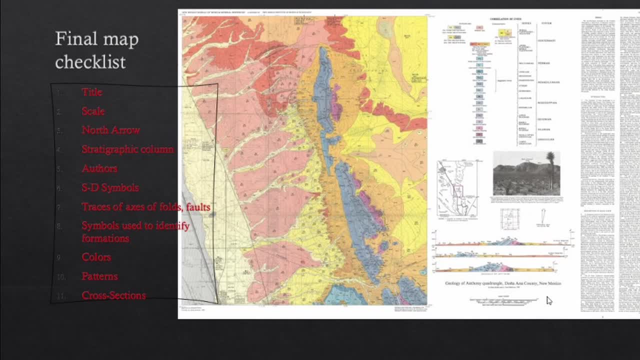 your authors, which I think this under the title Strike dip symbols. It's not zoomed in enough, but yes, there are strike dip symbols on this map. Traces of axes of folds and faults. I know that there's a fold right here in this area. It's a drag fold from a normal fault. Symbols used to 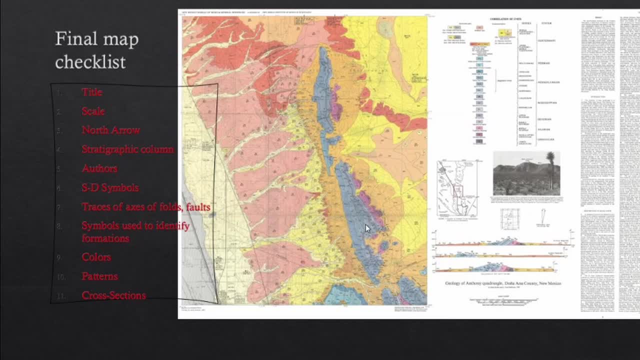 identify formations. Have these keyed to the map? Know what rock you're looking at when you're looking at your key and your map, Want to make sure the colors match each other, And then you want to be able to identify patterns in relation to your map, And then you have cross-section. 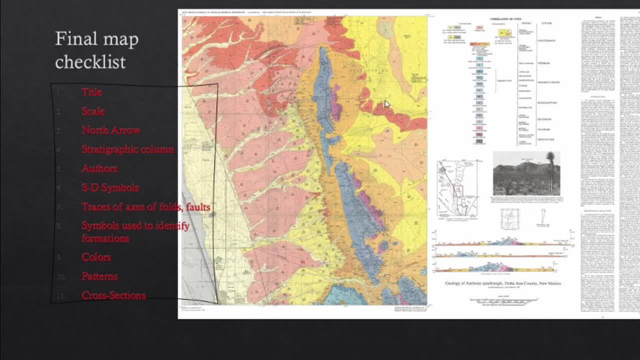 right here. There's three lines of cross-section: One right here, one right here and another one, one, two, three cross-section lines in this area, So let's hit the fill. Welcome back Essentials. We are here at the. 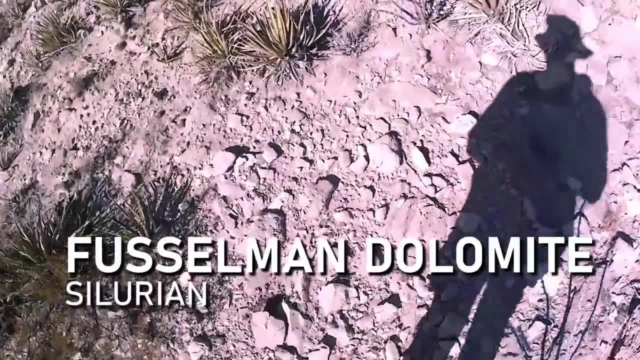 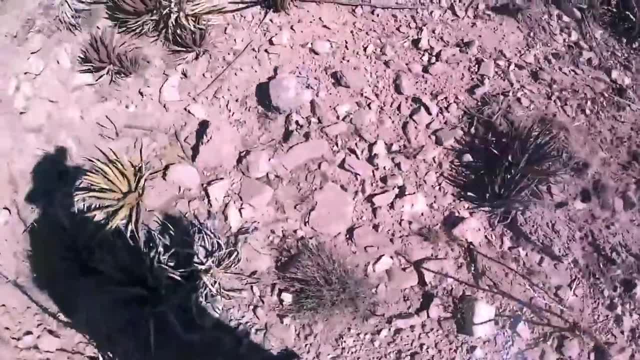 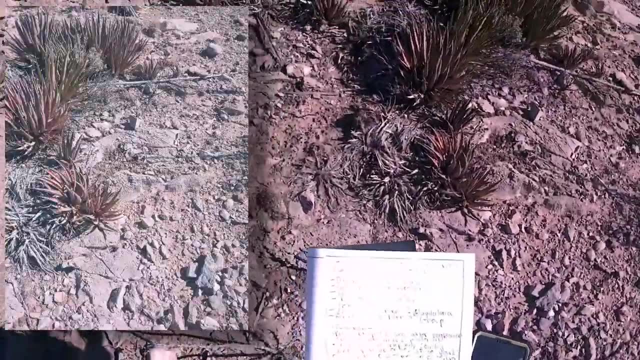 Fusselman Dolomite, And this is the first rock we're seeing here at Sierra Vista in New Mexico, Beautiful day. And so the Fusselman is a dolomite. It represents the return of an epiareic sea after regression. It's free of pterogeneous or land materials, such as sands, And it's thick. 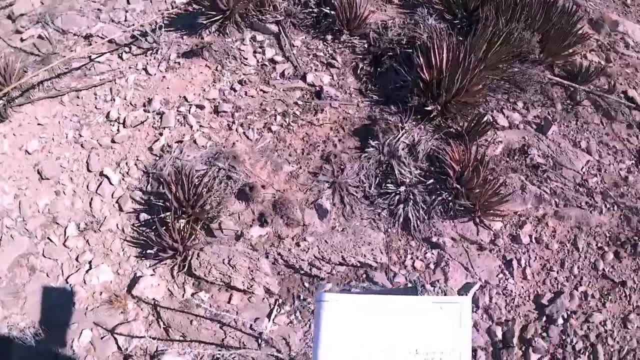 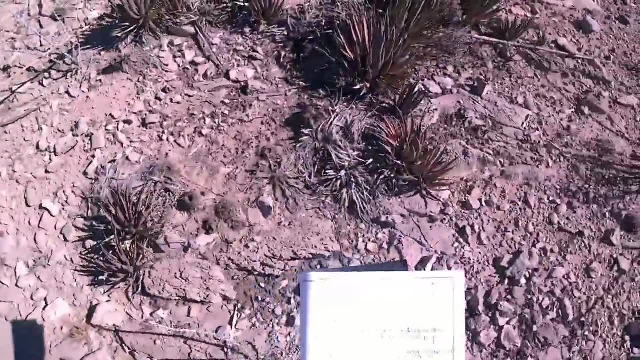 massive and complexly jointed. It's almost pure dolomite. It's white to dark gray. Its particles are 0.2 to 1 millimeter in size And it's even-grained, which means it's microtic It. 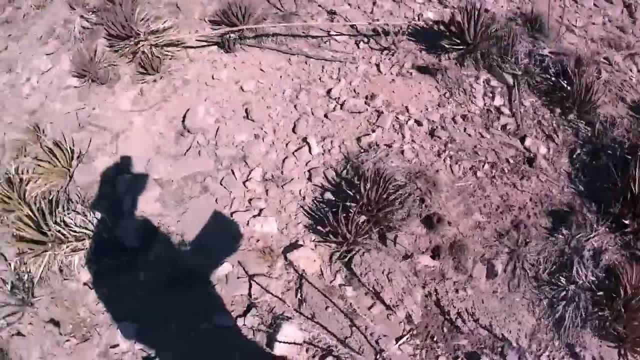 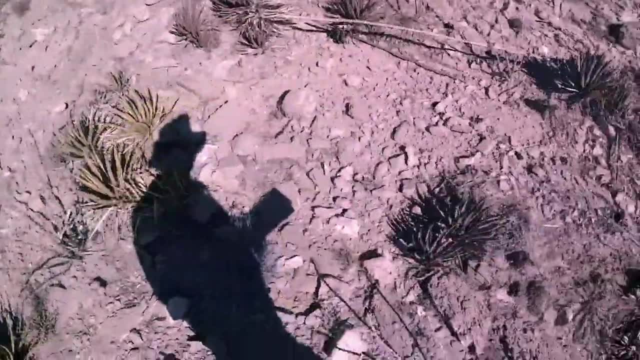 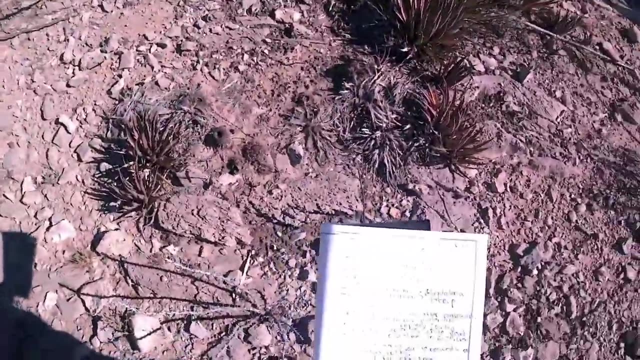 weathers brown, with vein-like networks of chert and chert nodules, And it was deposited far offshore in a shallow sea. Corals are a common fossil you'll find here in the Fusselman, And the corals represent a warm, shallow sea. That's where they lived during the Paleozoic And you have a lack. 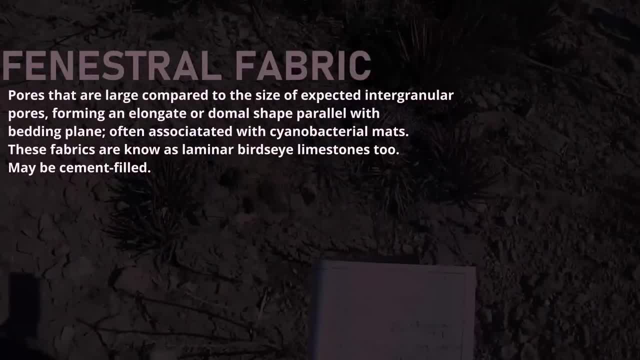 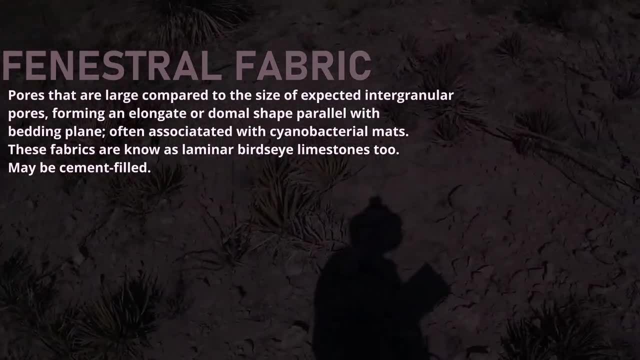 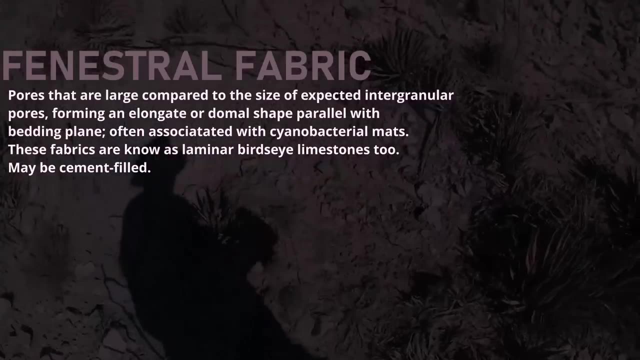 of detritus or land-derived materials, which is a common fossil, And it's a common fossil, And it's a calm sea or restricted circulation by reefs, And in some cases you can find stromatolites and bioherms. And another common characteristic of Fusselman is the fact that it has fenestral. 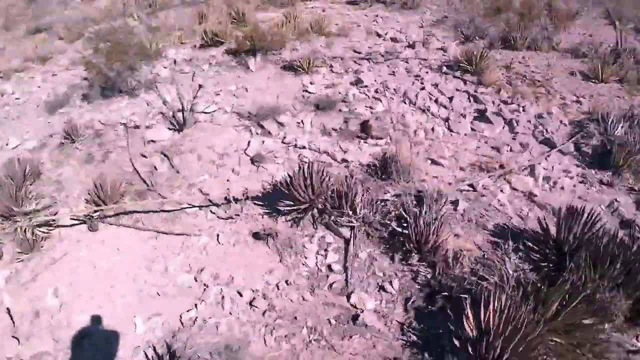 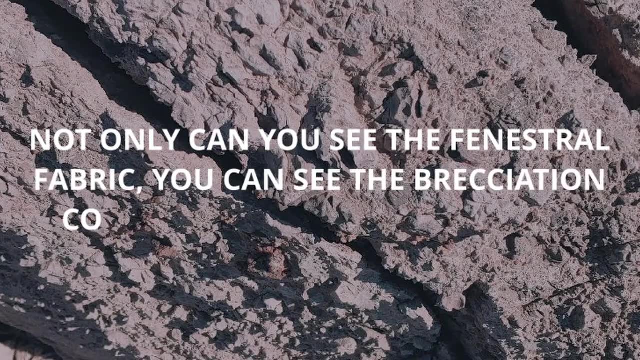 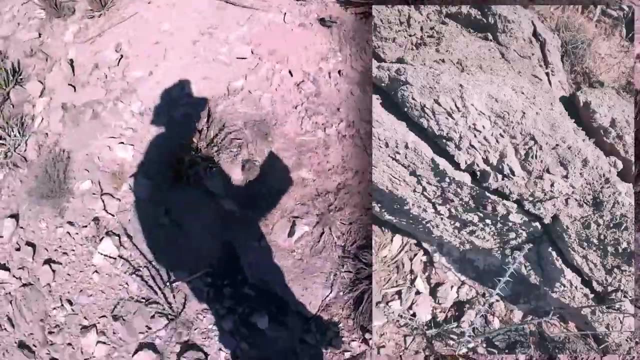 fabric- Fenestral fabric- is basically algal farts And they create these bubbles on the surface of the rock. At the time it wasn't a rock, It was sediment, But you had this algae basically putting it together And it created these bubbles And you can see that in this rock. And another thing is 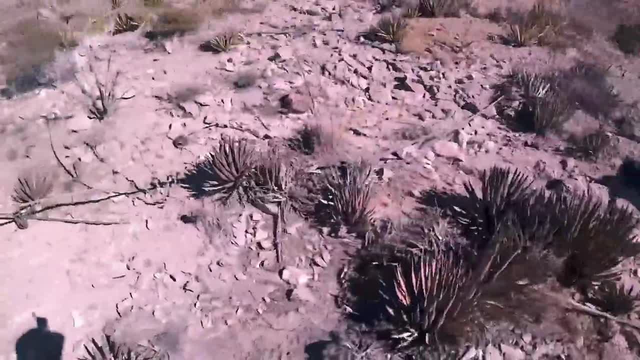 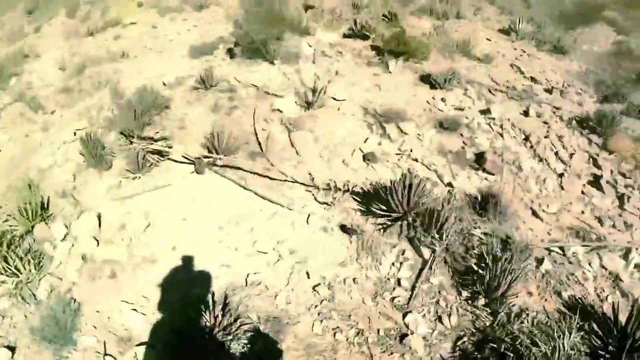 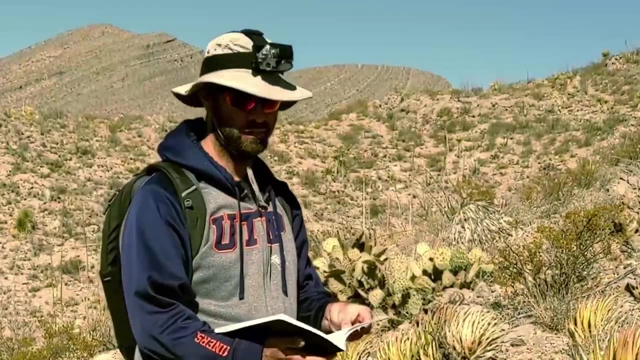 that some of this material was fragmented and then re-cemented together. So it has a very fragmented look to it. It's probably shattered- bioherms most likely- And then re-cementation occurred All right. So we're sitting on a normal fault, the large normal fault that cross-cuts this entire. 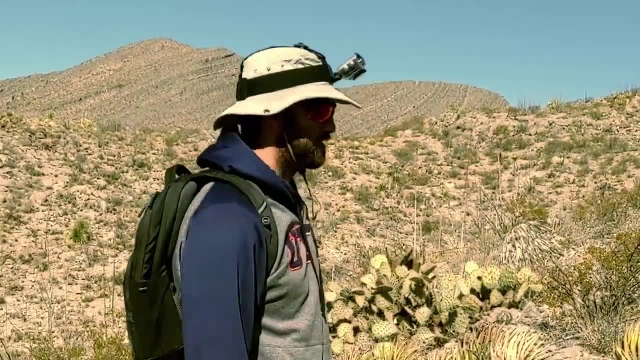 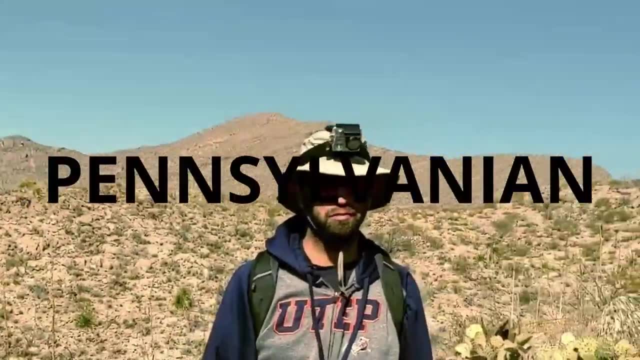 site. This is the burrino right here on your right side And we have the Fusselman down here. Those two should not be in contact with one another. One is from the Silurian, The other burrino is from the. That's a lot of geologic time missing. We're sitting on a normal. 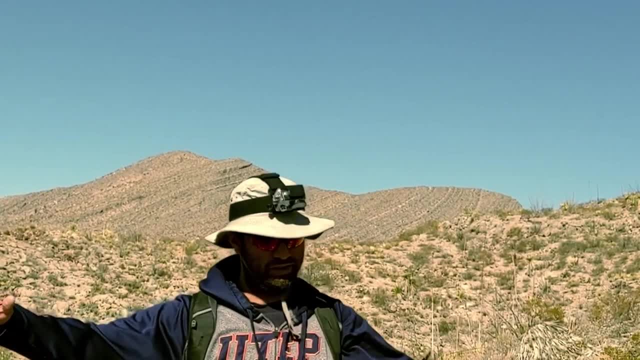 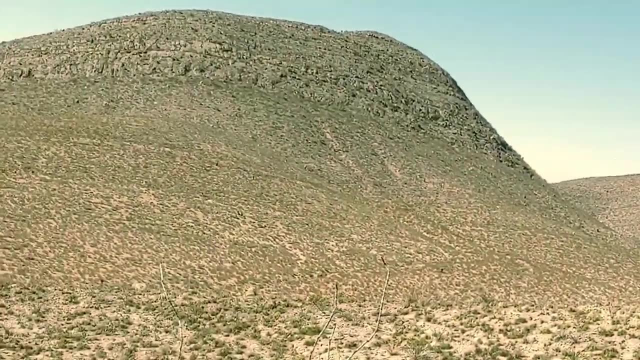 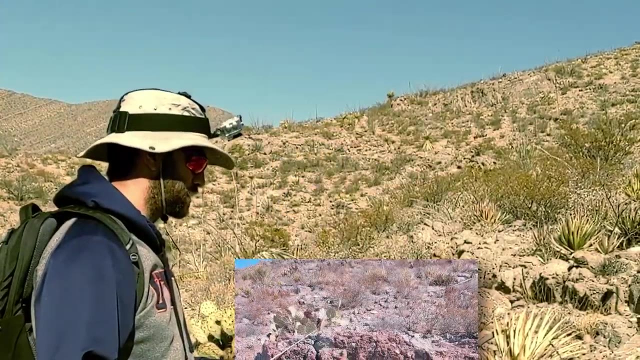 fault. right here You have the Fusselman and then the burrino, And obviously this is your uplifted block, down-dropped block, And then the burrino. in terms of the description you have, it's characterized by brown banded outcrop which you can see right here, Identical to the Latuna in. 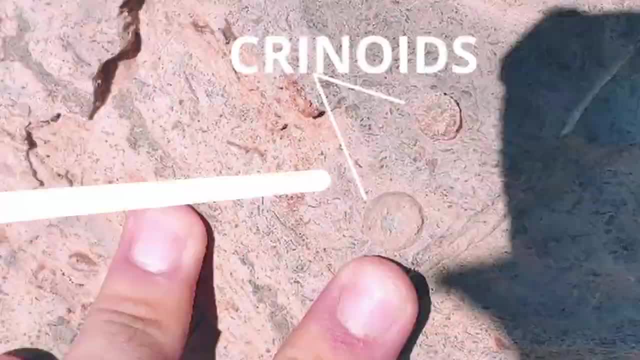 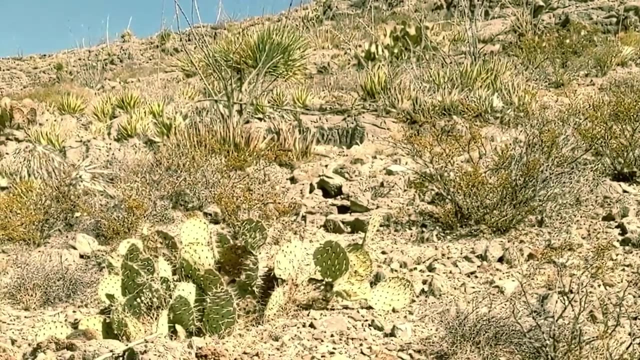 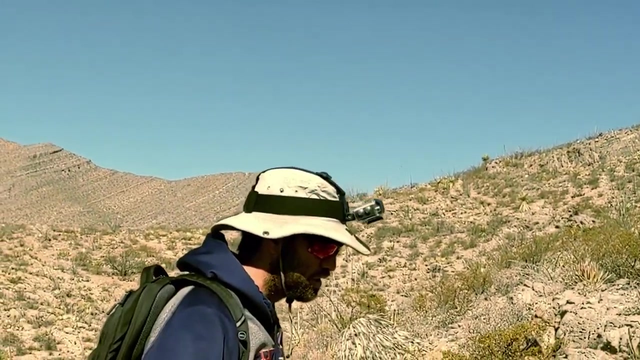 the sense that it's dense, crinoidal dark gray limestone with affinitic black chert nodules. This one actually can contain, in some places, wood fragments from trees being dropped into the ocean through erosion and being deposited with the limestone, which is pretty cool. And then you 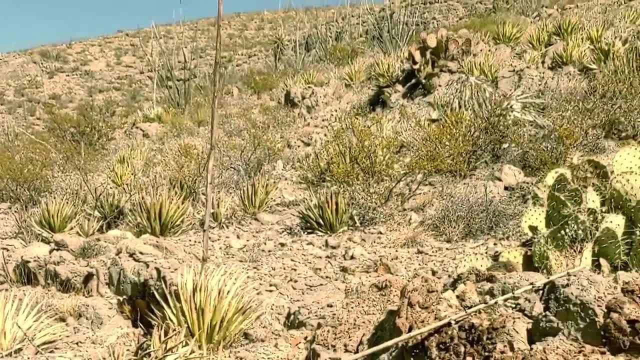 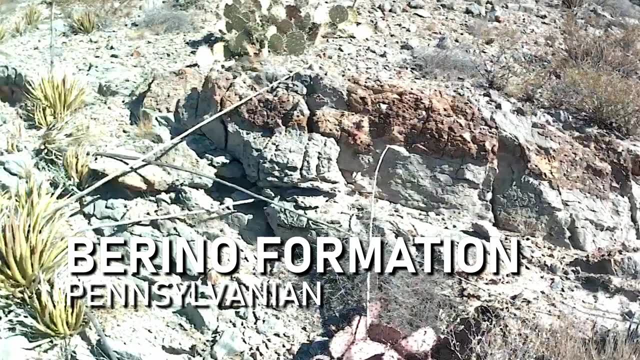 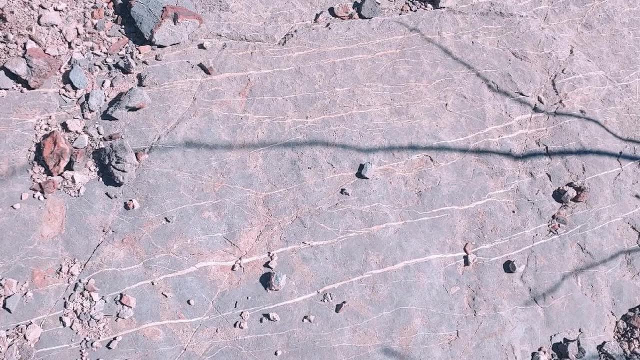 have alternating beds of shell and limestone with the burrino, And this is the youngest, youngest rock in the area. So, real quick, we were talking about structural analyses. I just have a picture of a vein array And that one that I mentioned in the previous episode, episode four. you can measure the width.